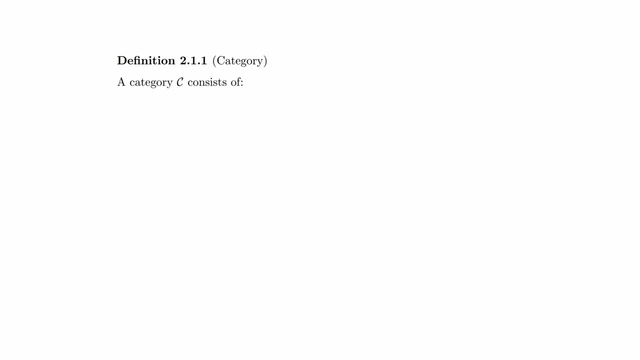 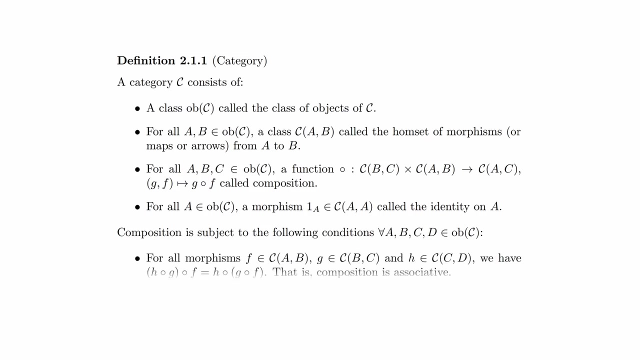 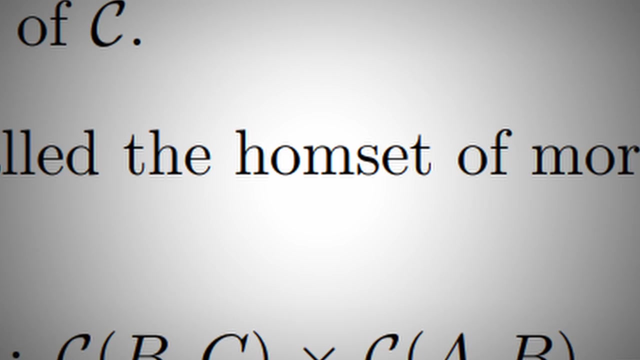 fact 2. A category consists of a collection of objects, for any two objects, a homset of morphisms from one to the other and a composition operation such that composition is associative and has identities for each object. Easy right- Fact 3. Not easy Homsets, Morphisms, The. 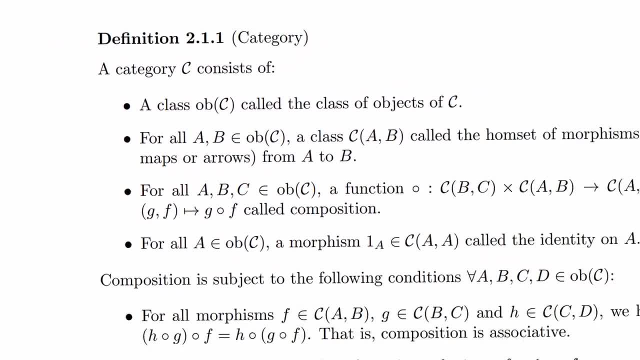 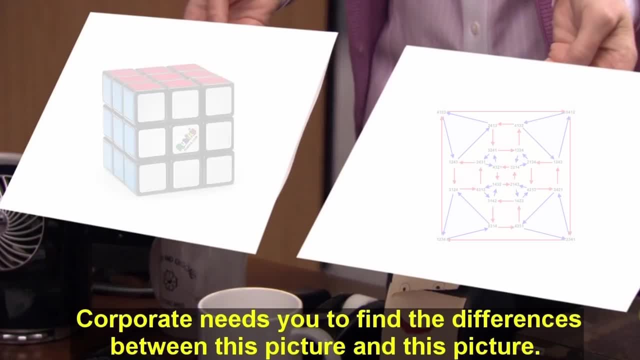 hell is an ob. You don't need any of those to understand category theory. No, you need that meme with two pictures that Pam from the office says are the same picture. That's all. mathematics is right. You take two things and find a theory that abstracts away their particulars to deal with them together. 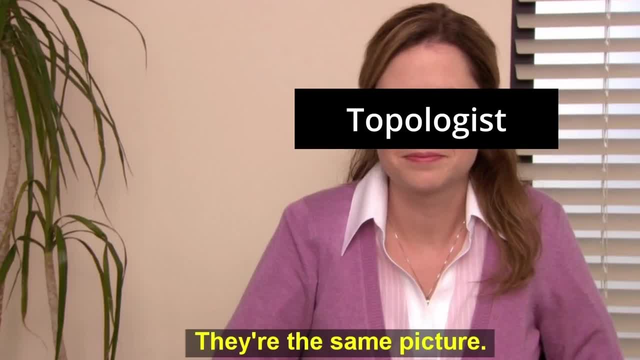 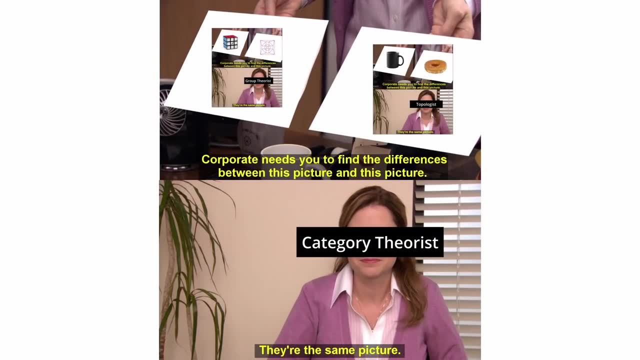 You know that whole thing about coffee mugs and donuts and how topologists can't tell the difference between them. Well, category theory does that. but meta To a category theorist: all of maths is the exact same thing In all constructions you have some kind of stuff. 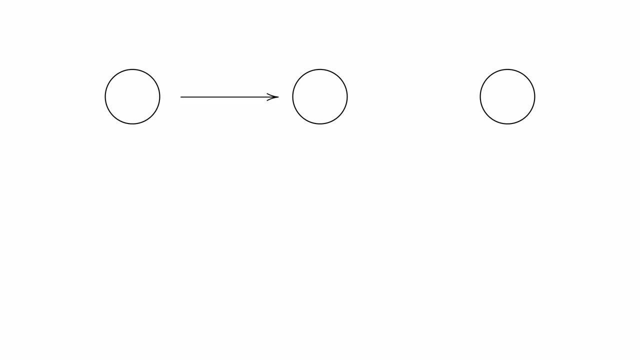 and stuff that relates that stuff, and you can chain those relations together to get further relations with the same properties. And sure you can call them objects and morphisms if you really want, but that's just gonna confuse people And we don't want to confuse. 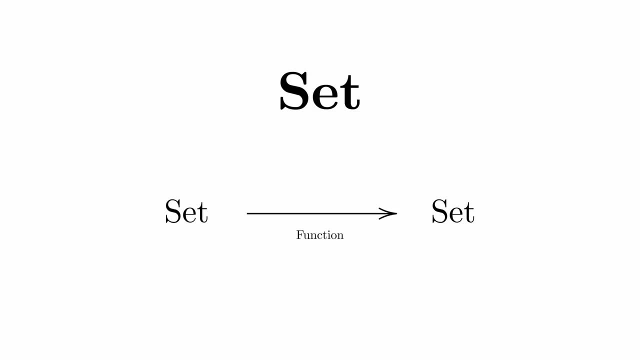 people right To that end. here are some illustrative examples: The category of sets and set functions, The category of groups and group homomorphisms, And the fundamental groupoid of a topological space where objects are points and morphisms are path homotopy. 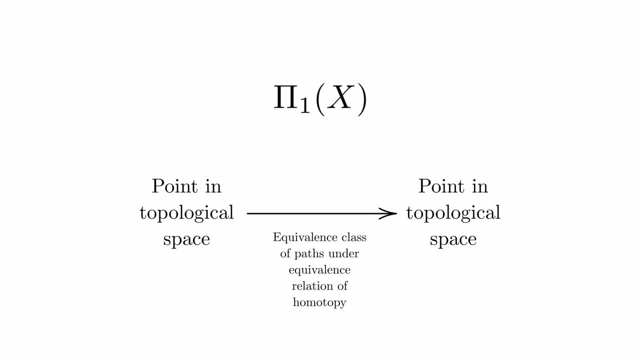 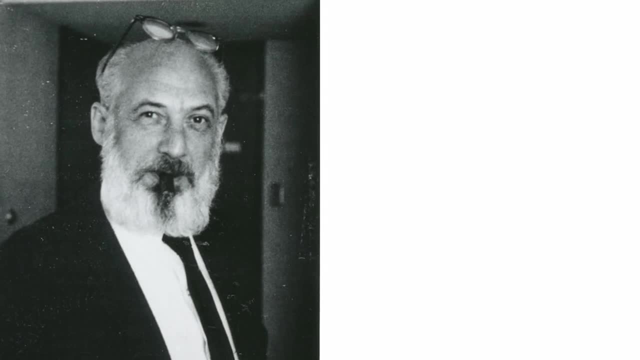 classes. And if you still aren't clear on what a category is after that, good luck. Fact 4. Category Theory was invented by American mathematicians Samuel Eilenburg and Saunders-McLean Mack Lane and officially appeared in mathematical literature for the first time in September. 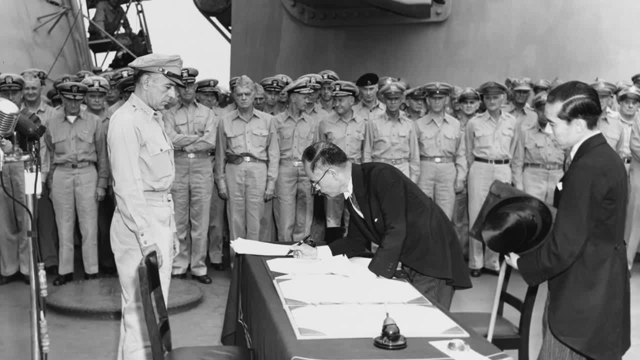 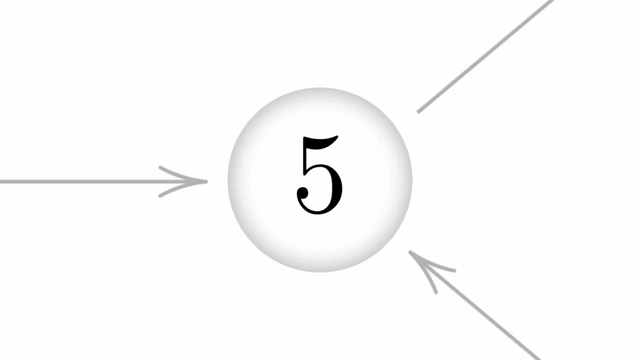 1945, coinciding exactly with the formal end of World War 2.. Category theory has been keeping the world safe from global conflicts ever since Fact 5. You can take some objects and morphisms from a category and arrange them to make a diagram. If all routes through the diagram, 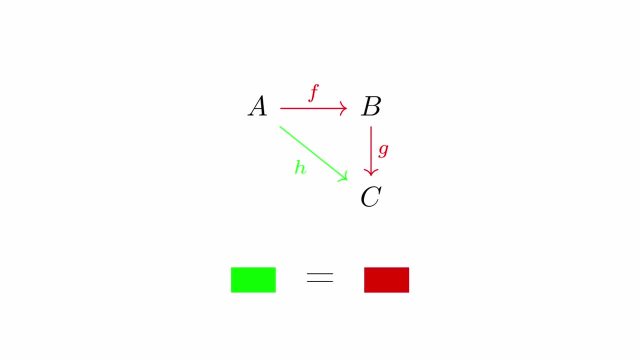 between the same two objects, evaluate to the same morphism. what you have? there is a commutative diagram. We say the diagram commutes. Commutative diagrams are equations for the category theorist. You thought a picture wasn't a proof? Well, think again. Commutative diagrams are everywhere Too. 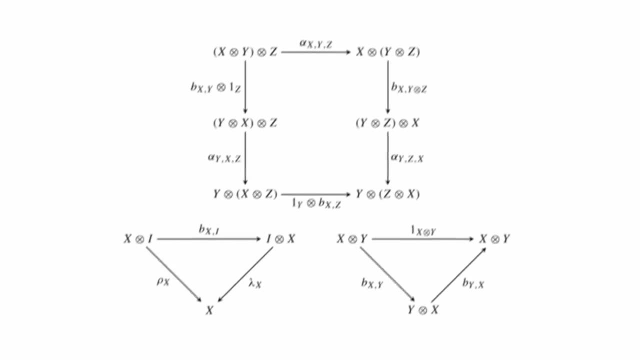 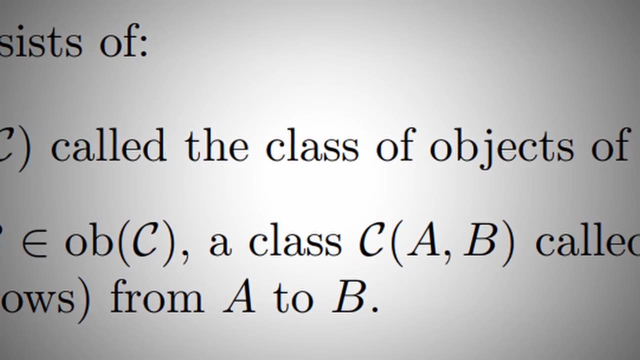 many places, probably. Alright, that's enough, Stop, Stop, Stop, Fact 6.. You might have noticed the word class in the definition of a category. You probably didn't, and that's okay. We all make mistakes. Why, though, use classes? 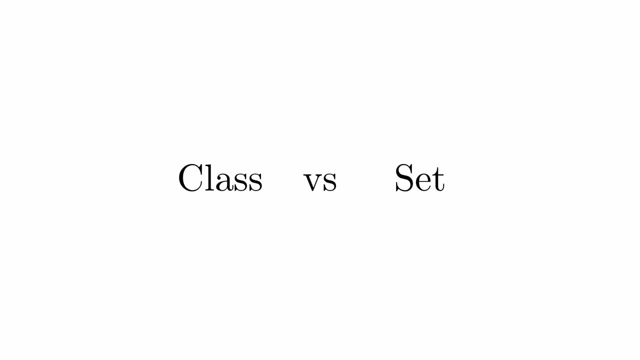 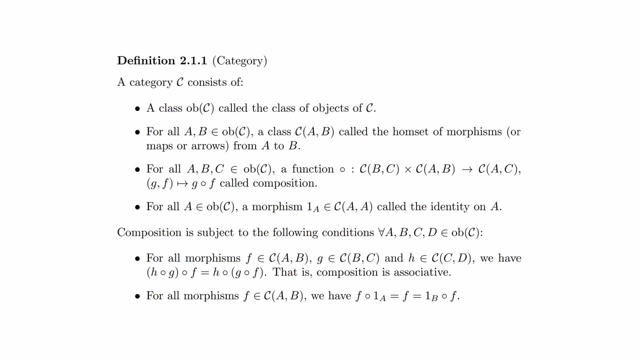 Classes rather than sets. Sets are nice and simple, Classes are weird and technical and annoying. In practice, almost everyone uses sets and ignores the distinction. We just put class in there to appease the set theorists, who would otherwise throw their paradoxes at us. It's a. 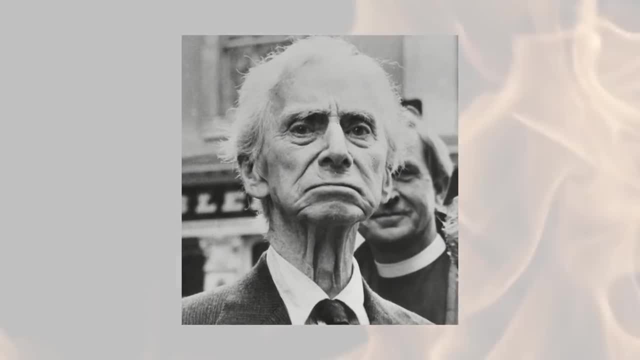 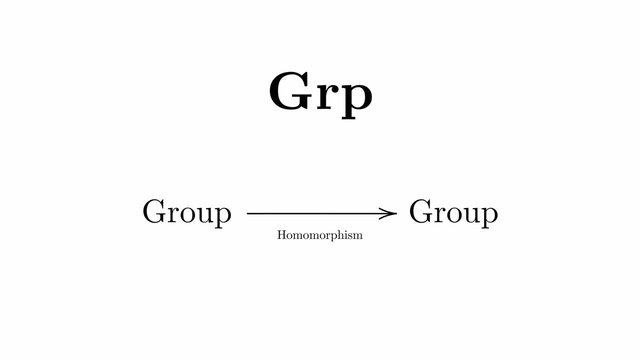 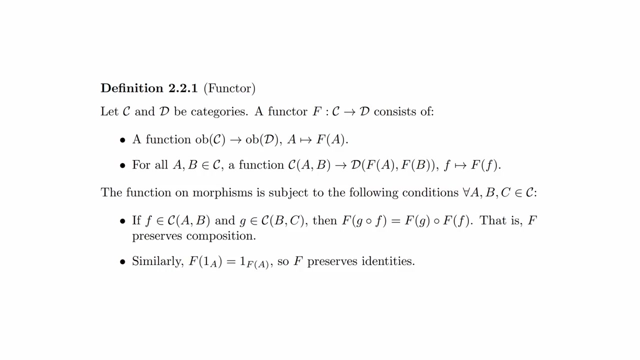 good idea to stay on the correct side of the set theorists. They can construct a set of all things that cause you pain. Fact 7. You can turn categories into other categories with functors. Yes, not function functor, One who functs. Functors take objects to objects and morphisms to morphisms. subject to sensible 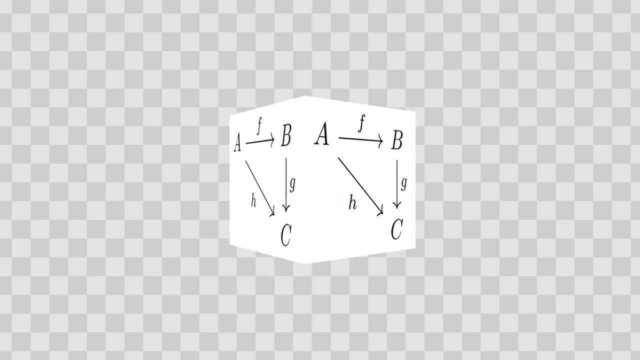 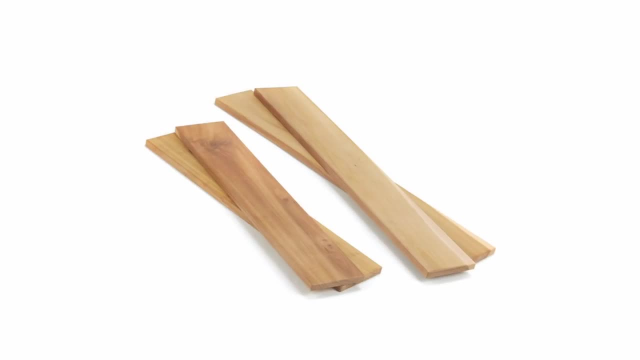 composition laws, But what that means for you is that they change your perspective on the world. You're looking at one thing, you apply a functor, and suddenly you're looking at something else. To use the meme analogy again, it's: uh, this one? Sure, Some of these functors are called. 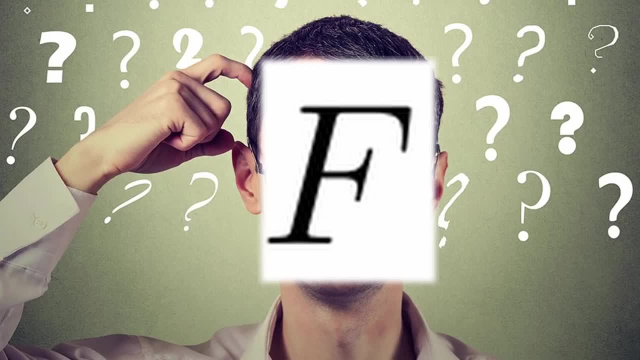 forgetful functors. They do nothing except forget some of the properties you cared about in the last category. A functor from the category forgetful is a functor that forgets some of the properties you cared about in the last category. A functor from the category forgetful is a functor. 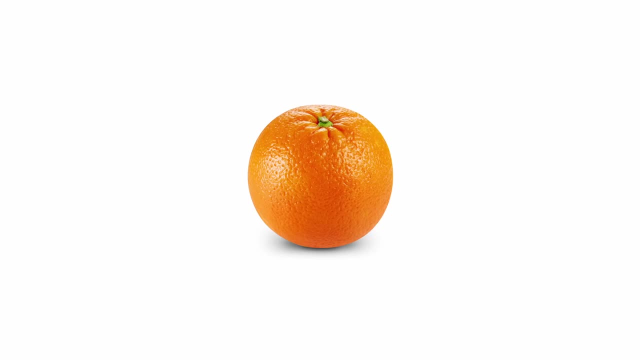 from the category forgetful, Because still we're listening to it. we're looking at the earlier one, Fact 8.. There are 5 ways to say things are the same in category theory: The same, basically the same, basically, basically the same, basically the same, but spicy and 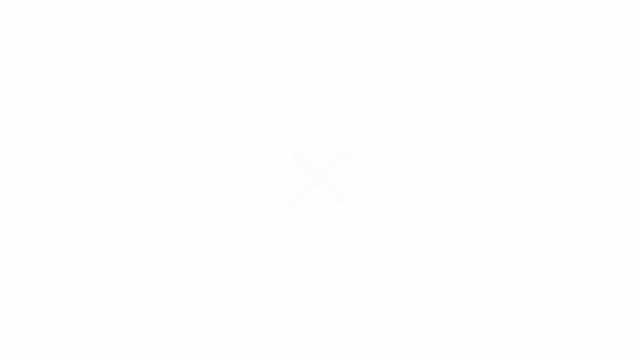 I don't even know how to explain this one. If you know any maths, you'll likely find lots of familiar words in category theory. But because we've abstracted beyond abstraction, they don't all look right. This is apparently a product, Yeah sure. 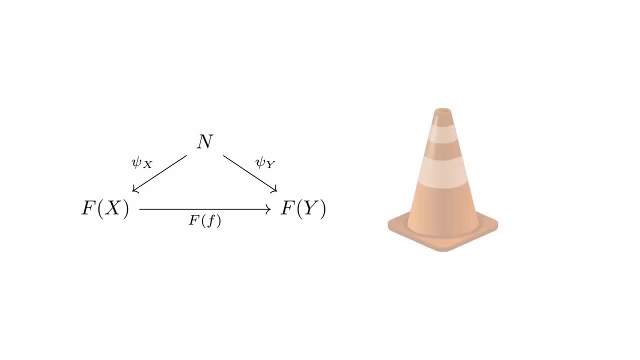 category theorists, whatever you say, And this, I'm told, is a cone. Hey, uh, Mac Lane, I think you need to go back to primary school, mate. This sort of thing does, however, mean you can study tensors without ever needing to know what a tensor actually is. You just need to understand. 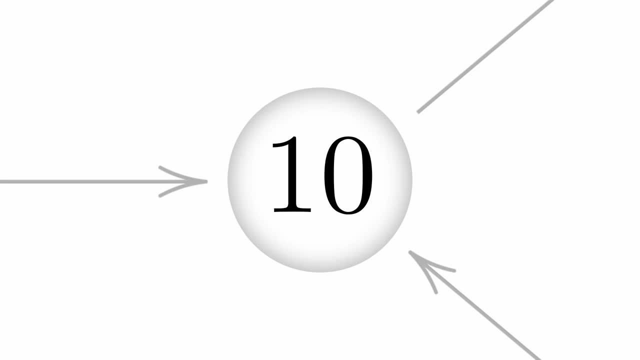 this commutative diagram Ha. Fact 10. The opposite of a functor is not called a defunctor. This makes me sad. Fact 11. You can do anything backwards by adding the prefix co. A backwards product is a coproduct, A backwards cone is a cocone, A backwards bra is a cobra, And I can't. 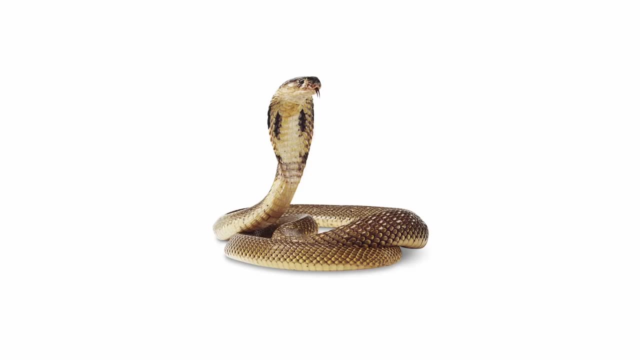 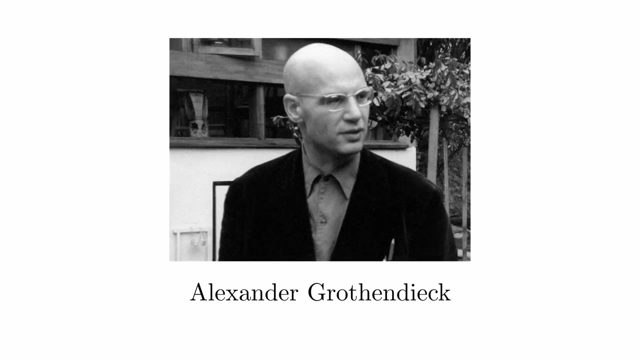 think of anything worse for support than a cobra. so the theory checks out. QED Fact 12.. One of the most famous category theorists was a guy named Alexander Grotendieck. Some people believe he's responsible for making category theory its own field of study, rather than a tool occasionally used in other. 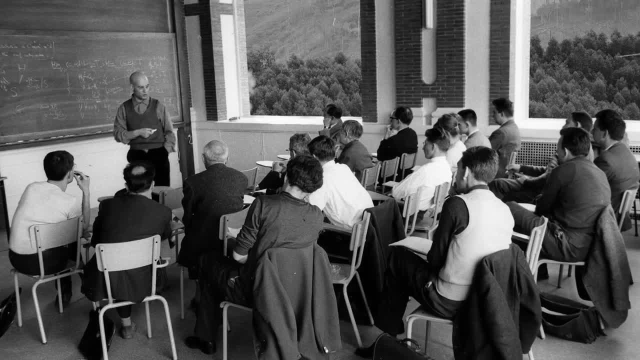 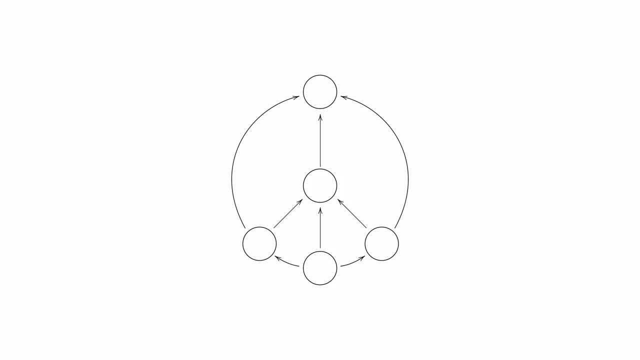 places. Grotendieck was a staunch pacifist and even gave a lecture on category theory in the forests surrounding Hanoi as it was being bombed during the Vietnam War. Once again, category theory is truly the ultimate tool for peace. Later in life, Grotendieck gave up on society. 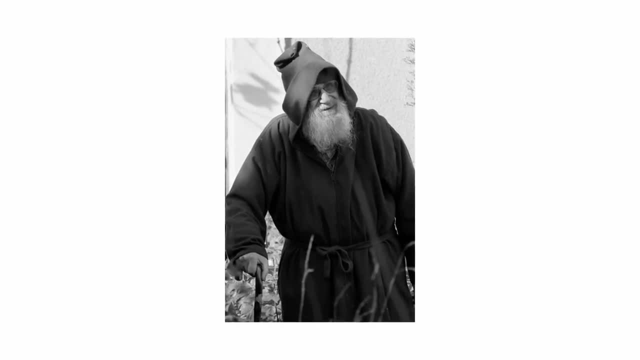 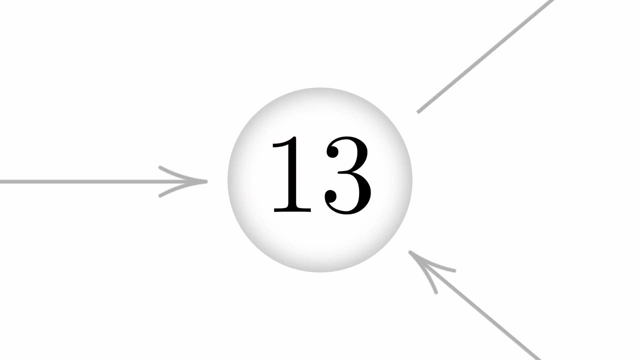 and went to live as a spiritual recluse in the French Pyrenees. He died in 2014,, but it's okay because his spirit lives on through the Twitter account, Grotendieck, Googling Fact 13.. Remember functors? They're maps between categories, But what about maps between functors? 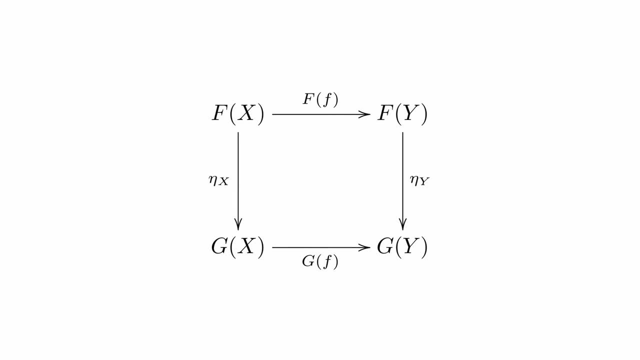 Mind blowing. I know right, These are called natural transformations. Natural transformations require that all diagrams of this form commute Simple Fact 14.. There's a thing called the Yennei Dilemma which says that if you know what a thing looks like from all perspectives, you know what it is. Students can get stuck flip-flopping. 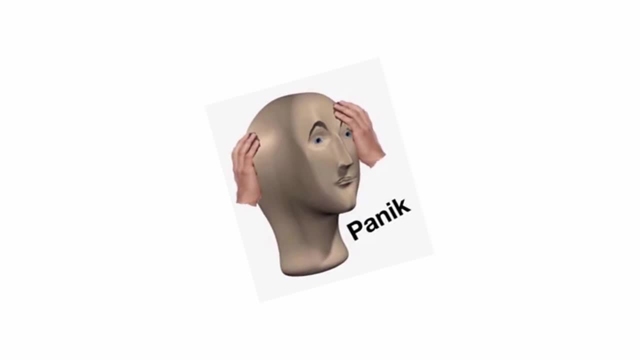 between believing the Yennei Dilemma is entirely trivial and believing it's the most complex thing they've ever seen. Fact 15. Remember natural transformations. They're maps between functors, But what about maps between natural transformations? You see the category of categories together. 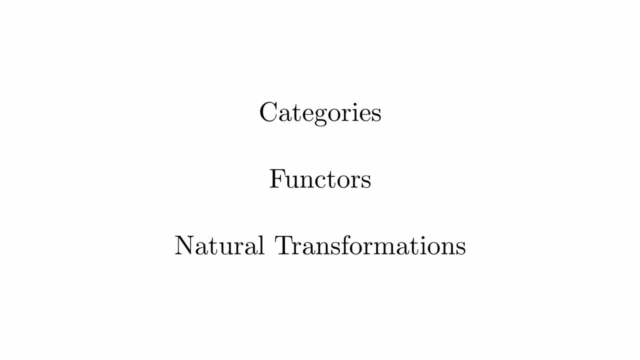 with functors and natural transformations is in fact an example of a two-category. These have objects, morphisms and morphisms between morphisms. Ah, but we've started counting now, and once mathematicians start counting, they can't stop. Literally, You've got your three categories, with morphisms between morphisms between morphisms. 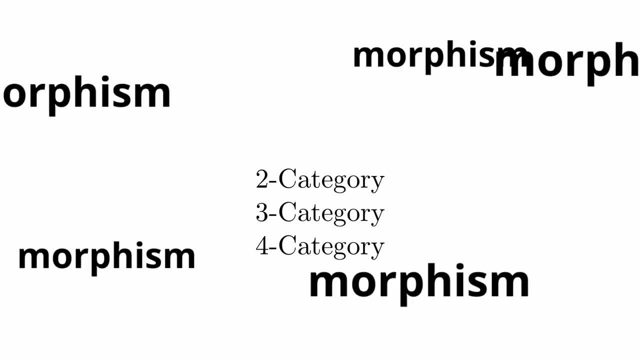 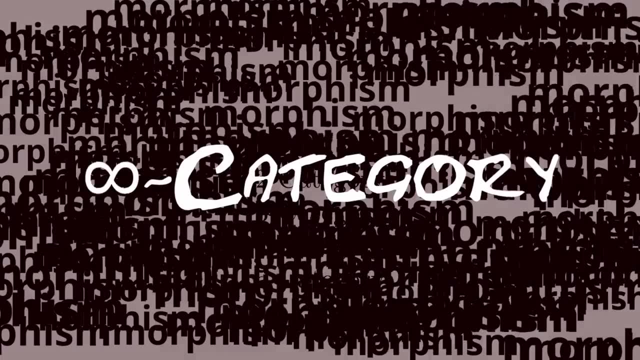 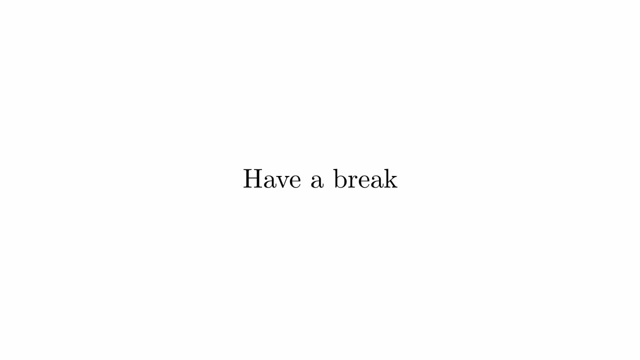 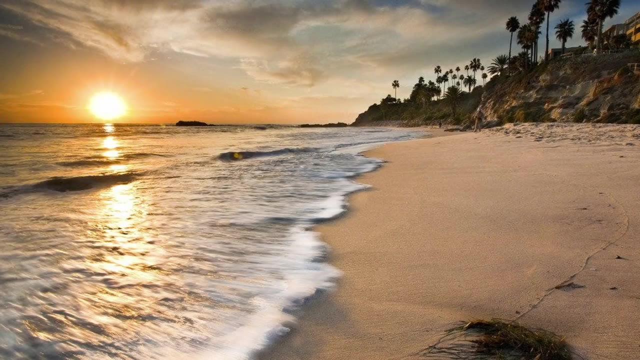 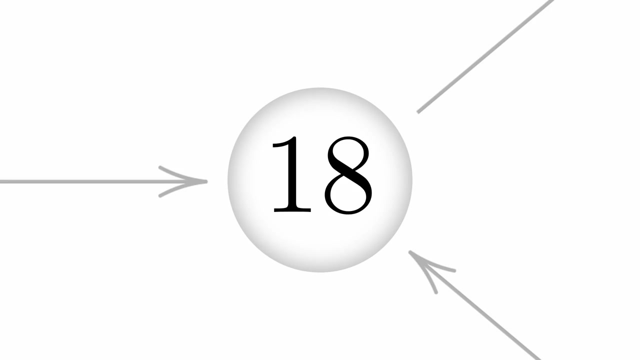 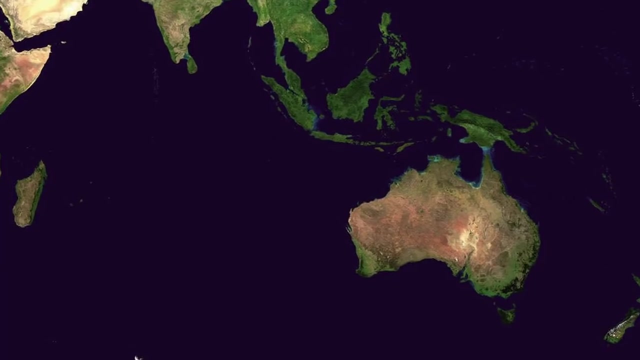 what the hell even are those Fact 16.. Have a break. Fact 17, a coconut is just a nut. Fact 18, due to its extended isolation from the rest of the world, Australian category theory has developed into a strange beast that even other category theorists fear. 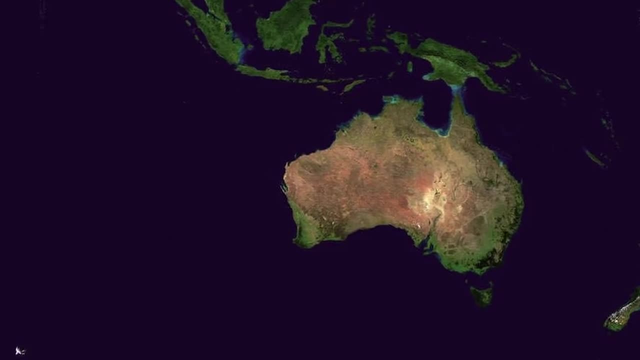 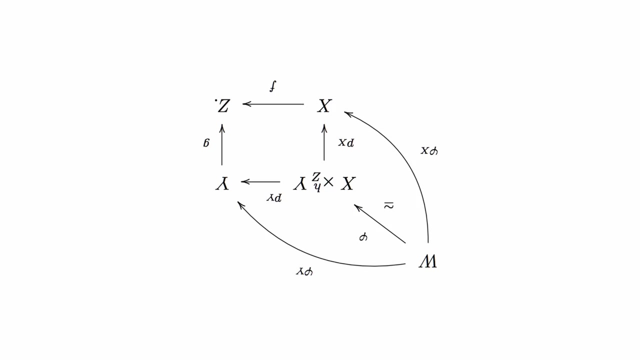 Its separate evolutionary lineage allowed it to reach levels of abstraction never dreamed of in the old world. So basically, it's the mathematical equivalent of marsupials. Also, all their commutative diagrams are upside down, Fact 19,. there's a thing called the pentagonator. 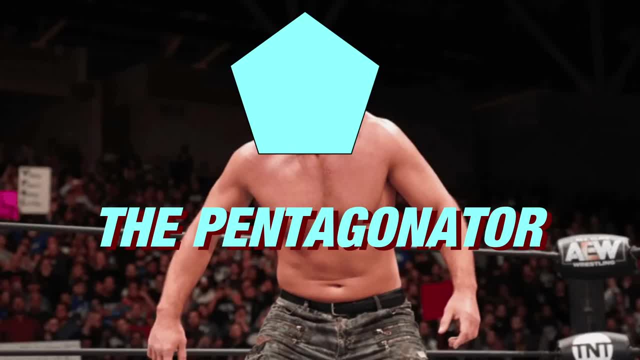 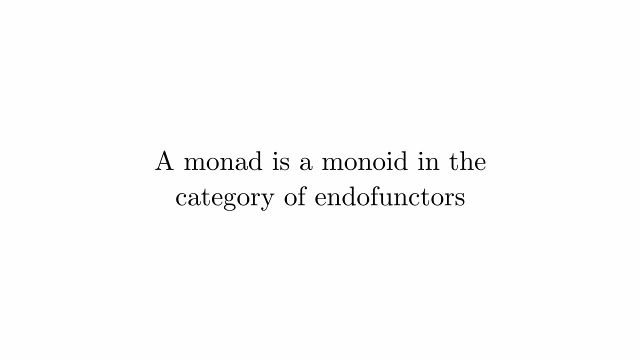 I don't really understand what it is, but knowing a word like that is out there somewhere makes me happy. Fact 20, a monad is a monoid in the category of endofunctors. Nobody actually knows what that means, so they'll just parrot. a monad is a monoid in: 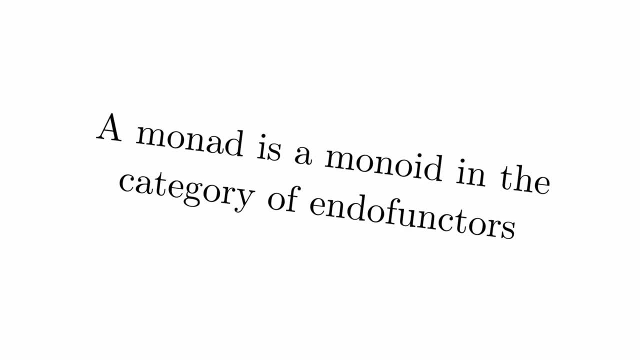 the category of endofunctors at you repeatedly to make themselves look smart. Fact 21, initial objects have morphisms to everything and terminal objects have morphisms from everything. Fact 22, category theory has lots of exciting real world applications. 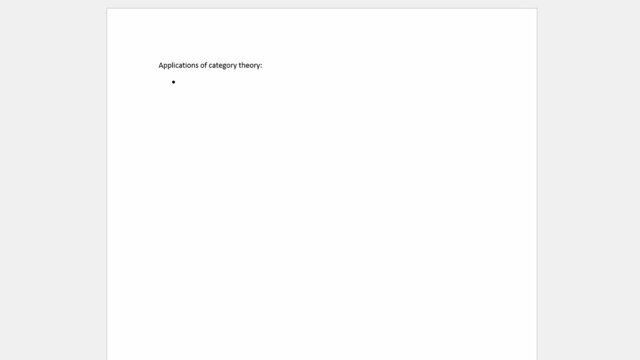 Such as: uh well, um, there's. there's a, I'm sure there was something. Fact 23,. what do you call someone who reads a paper on category theory A co-author? Fact 24, oh yeah, functional programming right. 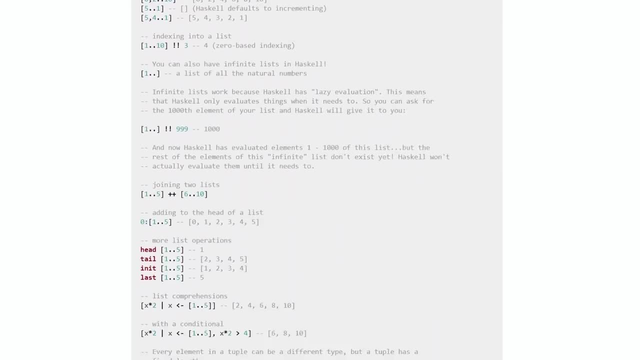 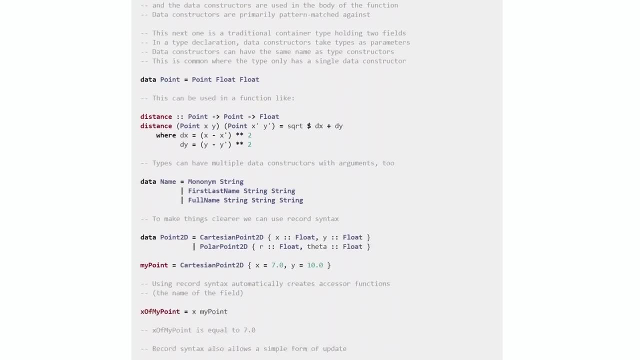 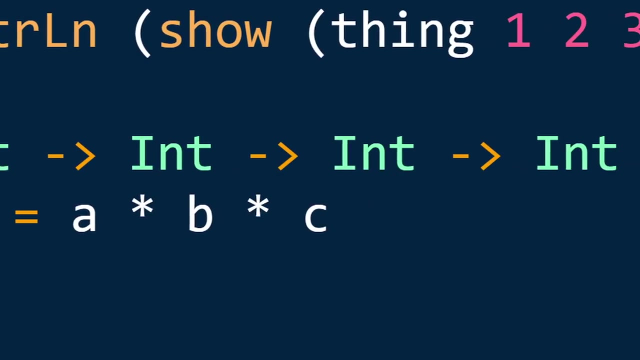 Functional programming is an increasingly popular programming paradigm that owes its development to category theory. Huzzah, we've found a real world application In functional programming. you pass functions as arguments to other functions And nothing keeps any state And you can have type: int to int to int to int. 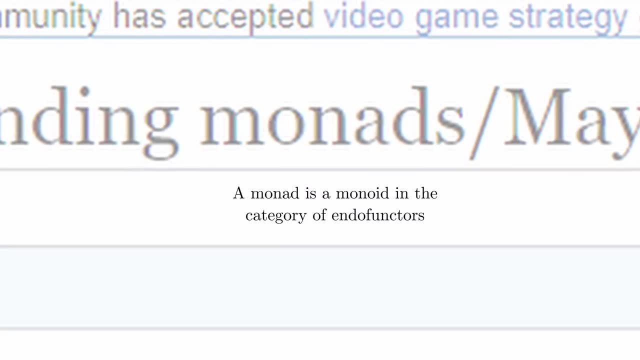 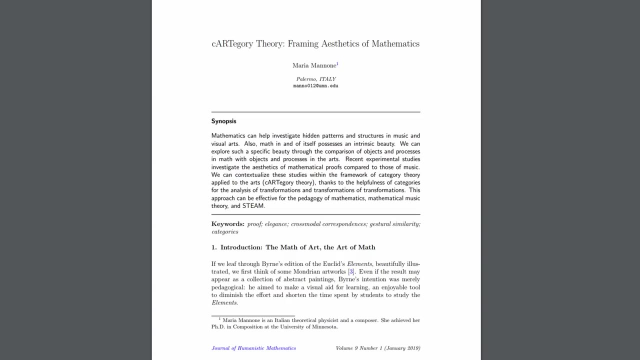 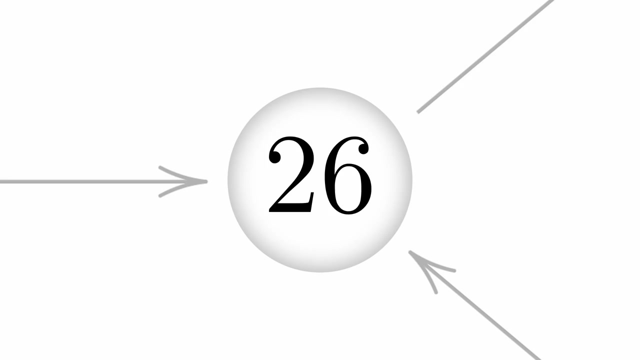 And there's this thing called maybe. Oh, how did that get in there? Fact 25, some people are tentatively applying category theory to the arts, art, music, literature, with a framework called ca-a-te-gory theory. Fact 26, in certain categorical constructions: